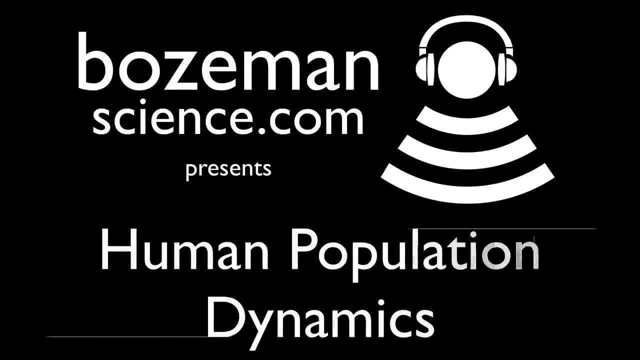 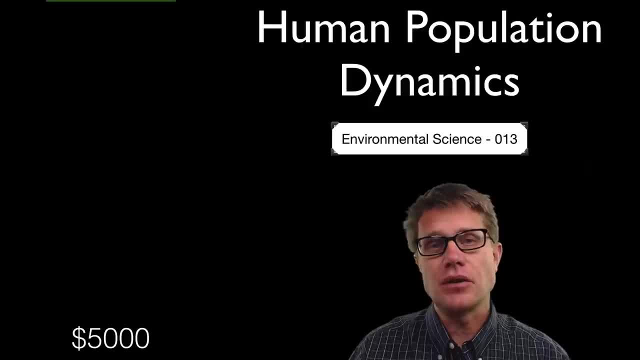 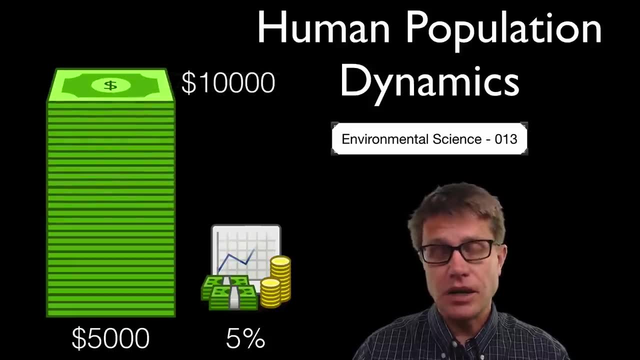 Hi, It's Mr Andersen and this is environmental science video 13. It is on human population dynamics. Imagine you had $5000 in the bank at 5% interest rate. How long would it take you to double your money to $10,000?? Well, you would have to go year by year. So it would. 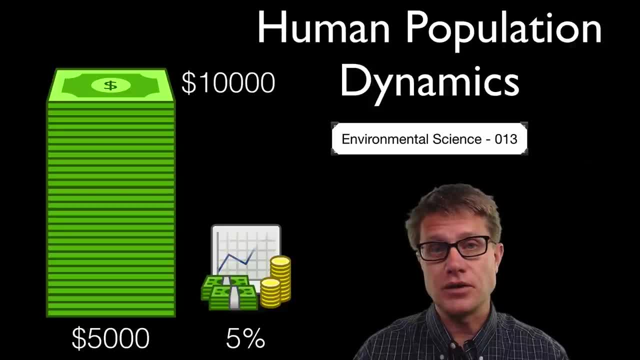 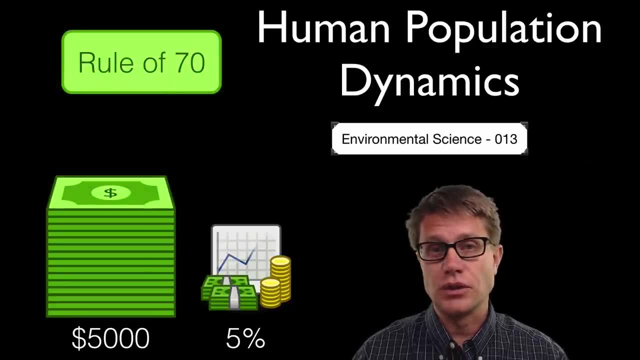 be 5000 times 5%, which gives you $250 in the first year. We would then have to take 5% of that and 5% of that. It is a really hard problem, Unless you understand the rule of 70,, which is really simple to figure out the time it takes to double your money all. 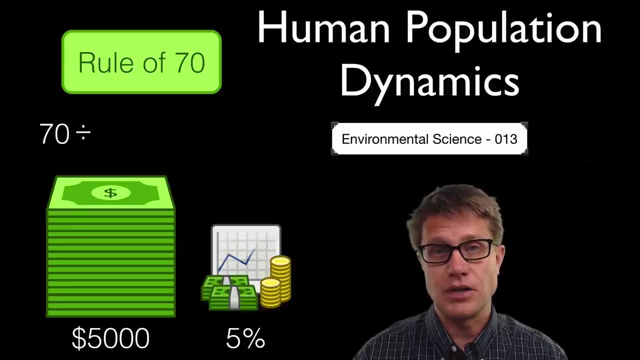 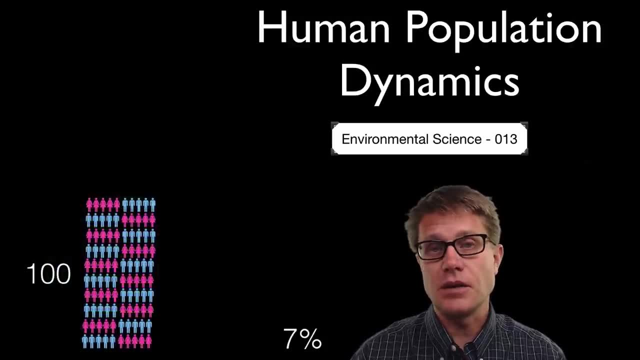 you do is take the number 70 and you divide it by that percent. So divide it by 5, and it is going to take you approximately 14 years to double your money. Super easy to do. Let's say we have a population of 100 individuals, A growth rate of 7%. How long is it going? 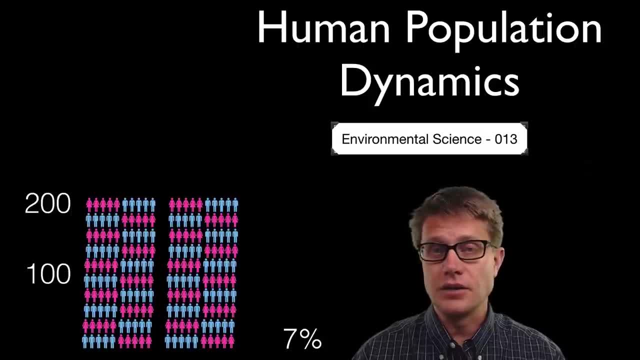 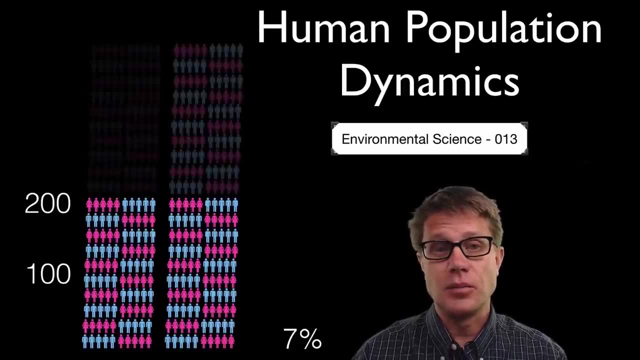 to take that population to double to 200 in size. All you do is take 70 divided by that growth rate. 70 divided by 7 gives you 10 years. How long is it going to take you to double it again, from 200 to 400? It is going to take another 10 years. And so you start. 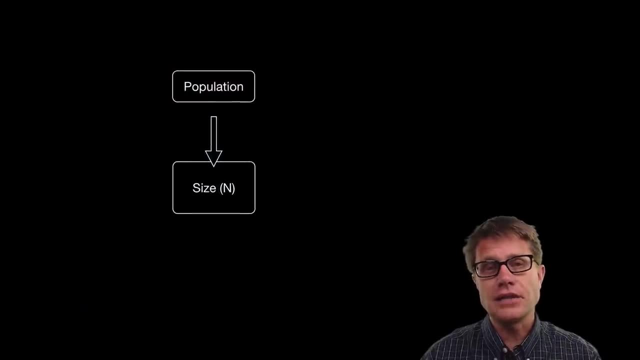 to see this exponential growth of the population over time. So in the last video we talked about the important characteristics of a population: The size which can be increased and decreased. We then talked about other characteristics: density distribution, age structure, sex. 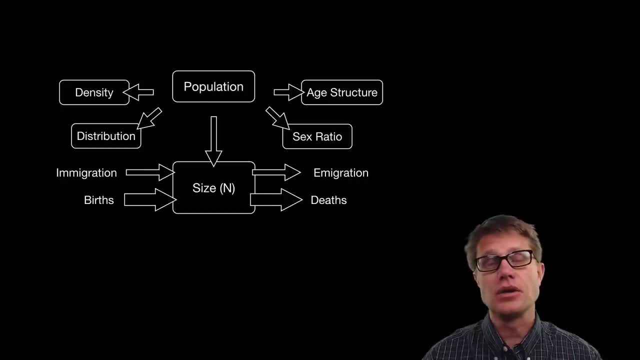 ratio. So in this video we are going to talk about how this all applies to the human population. We will start with density and distribution. We will then talk about the size and how that size has changed over time. It is very easy to calculate growth rate, And now you know how to calculate the doubling. 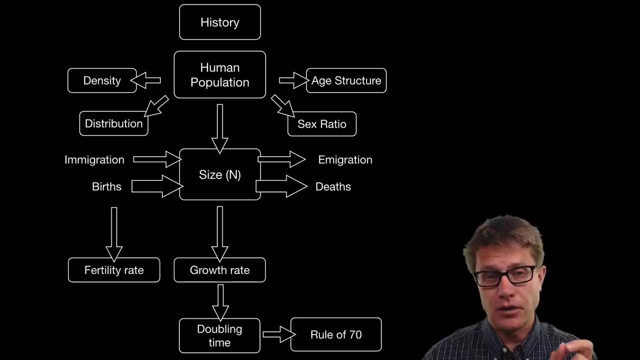 time using the rule of 70. We will talk specifically about birth rates using the fertility rate and death rates using the mortality rate, And then how industrialization, so the development of a country, can lead to what is called the demographic transition. And then, finally, we 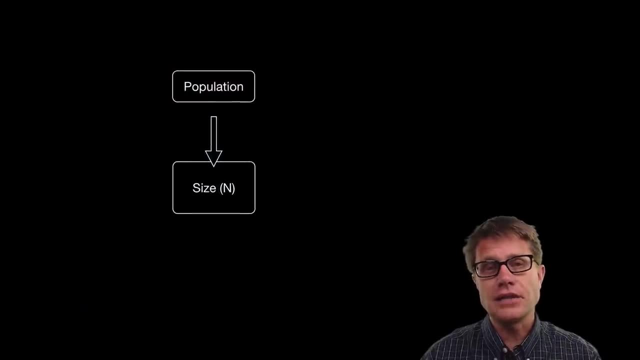 to see this exponential growth of the population over time. So in the last video we talked about the important characteristics of a population: The size which can be increased and decreased. We then talked about other characteristics: density distribution, age structure, sex. 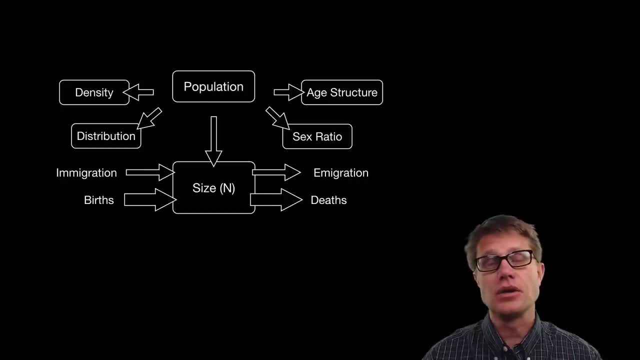 ratio. So in this video we are going to talk about how this all applies to the human population. We will start with density and distribution. We will then talk about the size and how that size has changed over time. It is very easy to calculate growth rate, And now you know how to calculate the doubling. 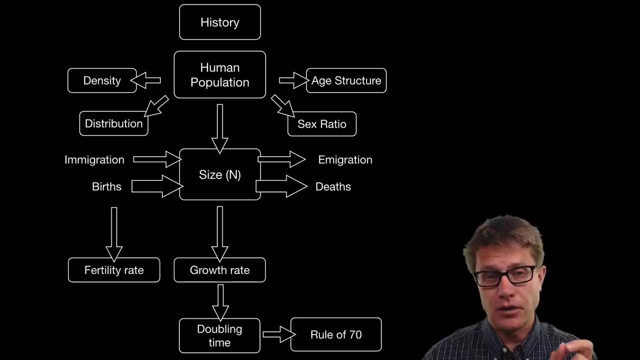 time using the rule of 70. We will talk specifically about birth rates using the fertility rate and death rates using the mortality rate, And then how industrialization, so the development of a country, can lead to what is called the demographic transition. And then, finally, we 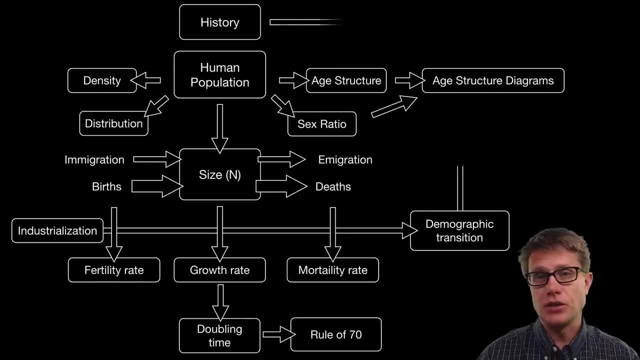 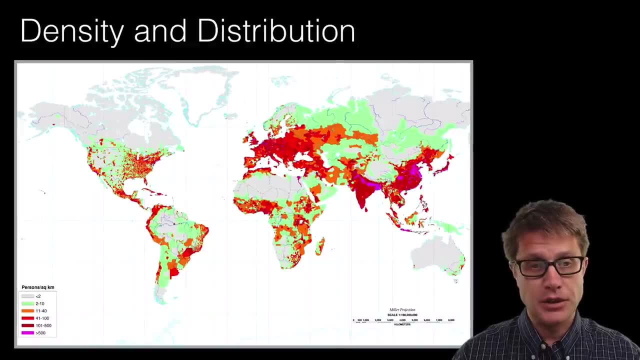 will finish up with the age structure diagrams, And these two things can be used as tools to predict the future population. And so if we start with human density and distribution, it is all over the place. So if we look here in Montana, it is less than two people per kilometer. If we look in the 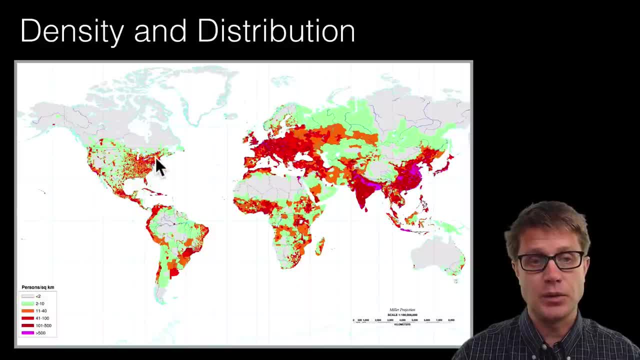 US. there are going to be way more people on the coasts, way more people in the Northeast, way more people in Western Europe and way more people in Southeast Asia. In certain areas it is going to be more than 500 per square kilometer, So there is unequal density. 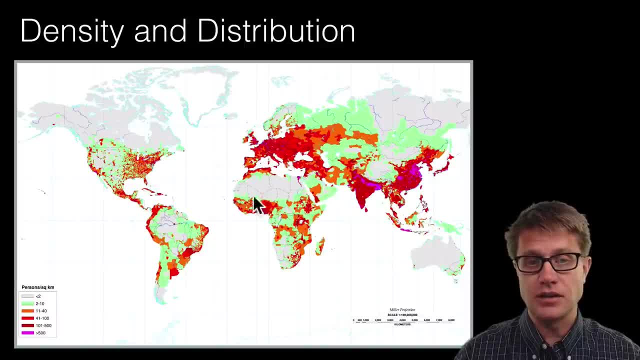 and distribution. You can also see some neat patterns. where there is desert, obviously there is not going to be a lot of people. We could look at the history of humans, which has maintained stability over a long period of time, So we can see that the population 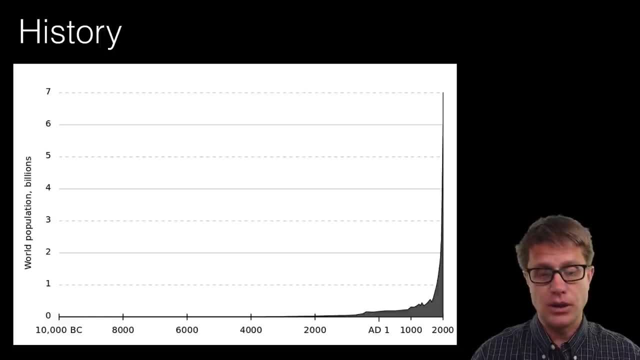 has increased in weight. And then you look at the history of humans, which has maintained time but recently has shown exponential growth. Now what led to that is going to be industrialization. So if you have access to constant food, constant sanitation, good medicine, we see an increase. 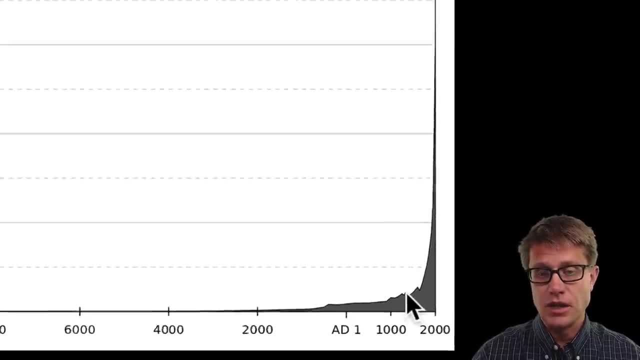 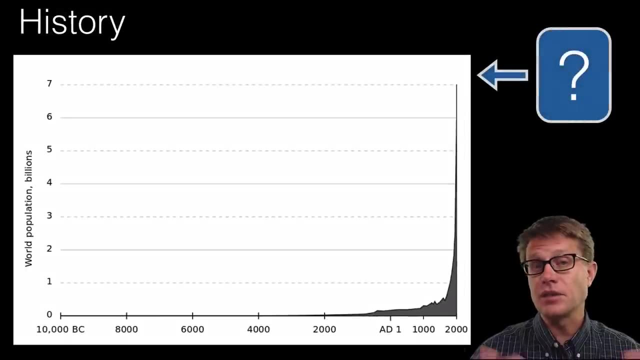 in the population. Now there are some blips along the way. There is going to be the bubonic plague, where a third of the people in Europe died, But you can see over time we are seeing massive increases. What happens next? We will talk more about that in the next video And 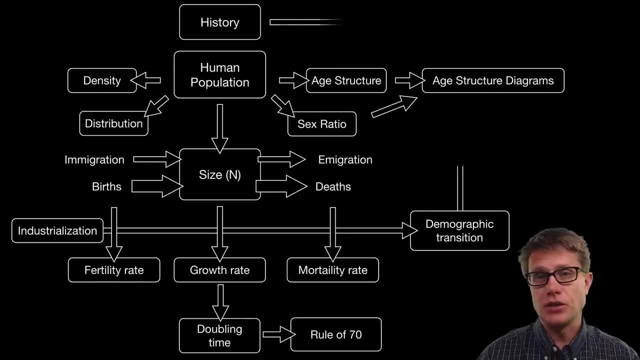 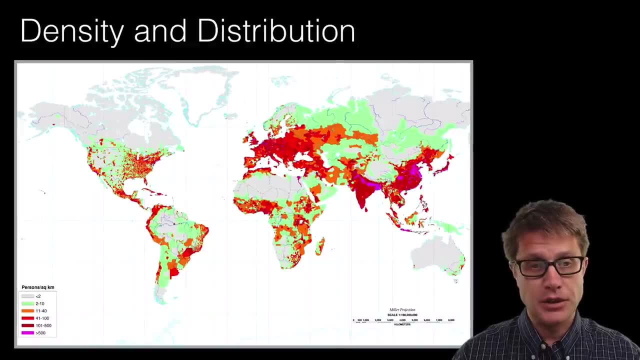 will finish up with the age structure diagrams, And these two things can be used as tools to predict the future population. And so if we start with human density and distribution, it is all over the place. So if we look here at Montana, it is less than two people per kilometer. If we look in the 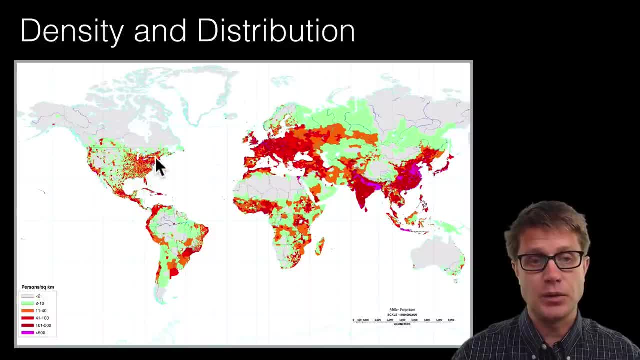 US. there are going to be way more people on the coasts, Way more people in the northeast, Way more people in western Europe and way more people in southeast Asia. In certain areas it is going to be more than 500 per square kilometer, So there is unequal density. 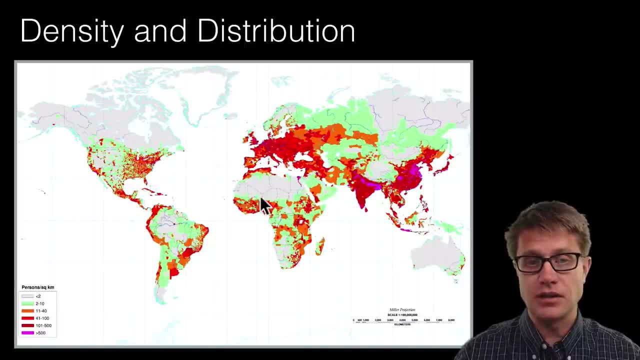 and distribution. You can also see some neat patterns. where there is desert, Obviously there is not going to be a lot of people. We could look at the history of humans, which is how it has maintained stability over a long period of time. PETER, so that will be. 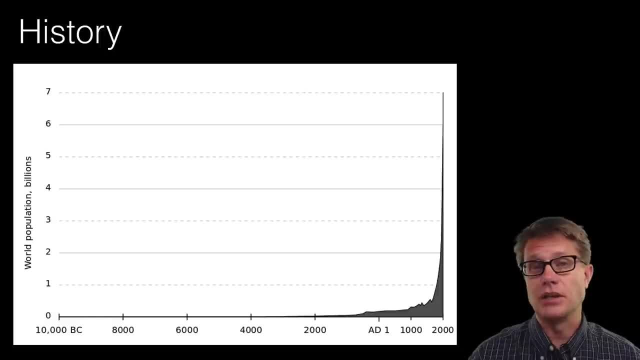 a couple resilience questions. So what we want to do is I am going to create an example which will you draw the world's first population. with regards to this population, And then we'll time- but recently has shown exponential growth. Now, what led to that is going to be industrialization. 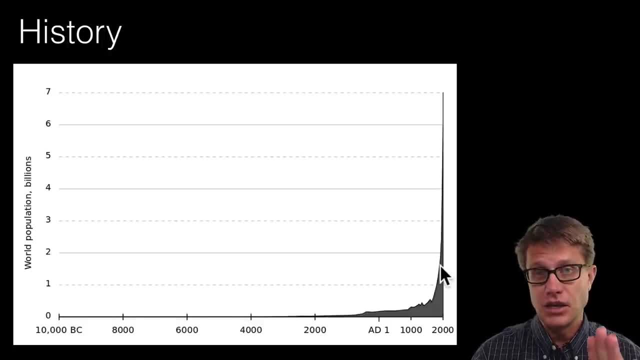 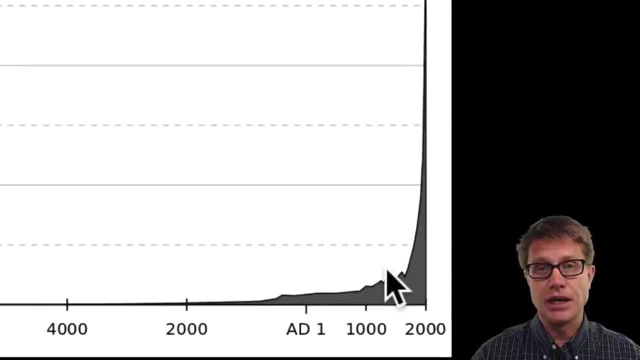 So if you have access to constant food, constant sanitation, good medicine, we see an increase in the population. Now there are some blips along the way. There is going to be the bubonic plague where a third of the people in Europe died. But you can see over time. we are seeing 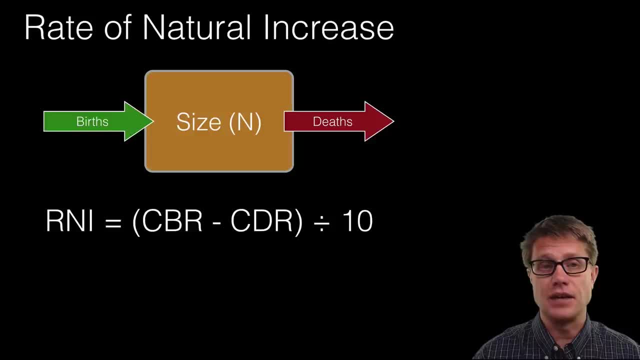 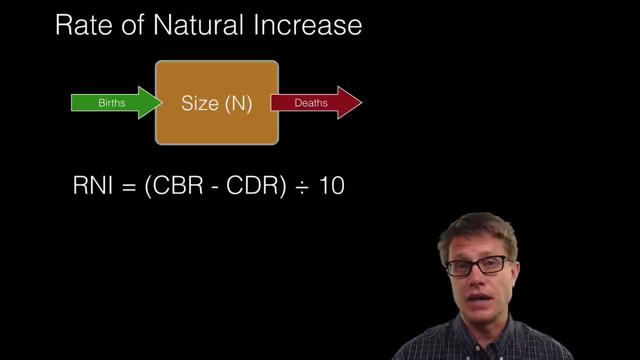 massive increases. What happens next? We will talk more about that in the next video. And so, if we look at the basic level, what is increase in a population Births, What is decrease in it Deaths, And so we have what is called the rate of natural increase, And 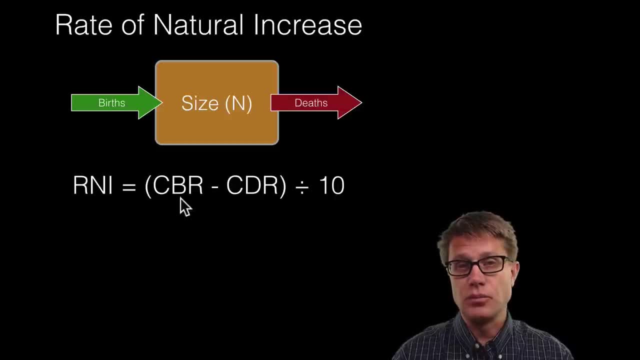 so the equation is simple: Rate of natural increase equals the crude birth rate minus the crude death rate, divided by 10.. And the reason we are dividing by 10 is these values are generally expressed per thousand people. So in 2013, the crude birth rate in Afghanistan: 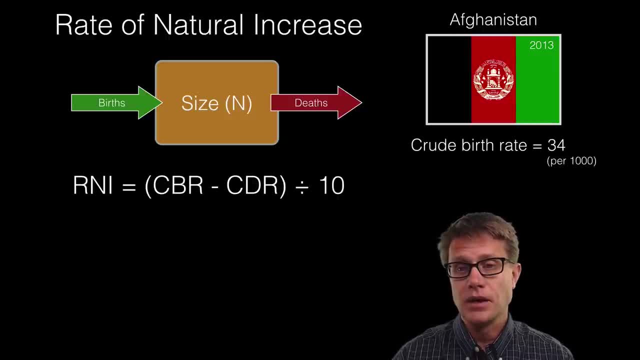 was 34 people being born for every thousand people. Crude death rate is only 8.. So if we want to figure out the rate of natural increase, we just plug those values in. 34 minus 8 is 26, divided by 10 is 2.6 percent, And so that means this population is going. 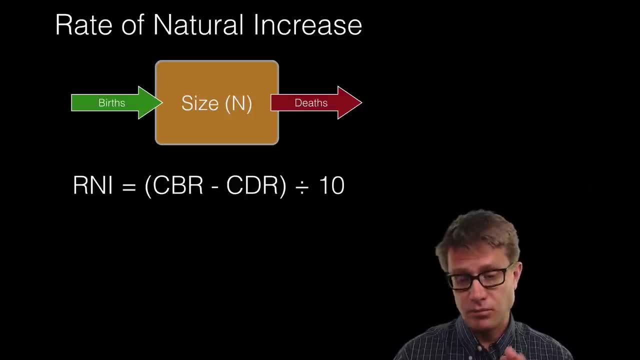 so, if we look at the basic level, what is increase in a population Births, What is decrease in it Deaths, And so we have what is called the rate of natural increase. And so the equation is simple: Rate of natural increase equals the crude birth rate minus. 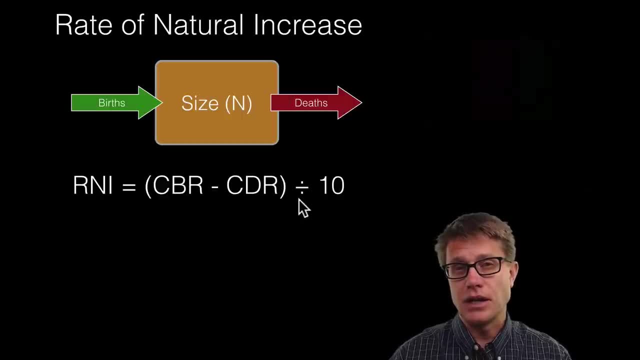 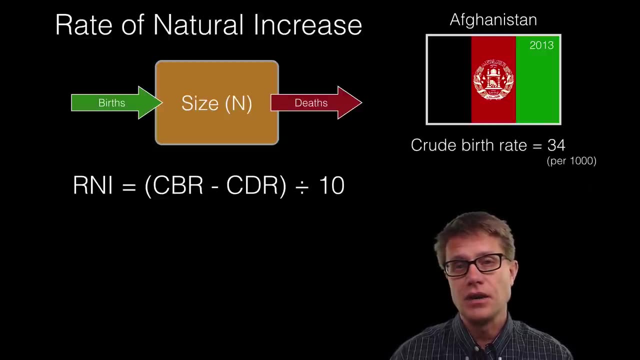 the crude death rate divided by 10.. And the reason we are dividing by 10 is these values are generally expressed per thousand people. So in 2013, the crude birth rate in Afghanistan was 34 people being born for every thousand people. Crude death rate is only. 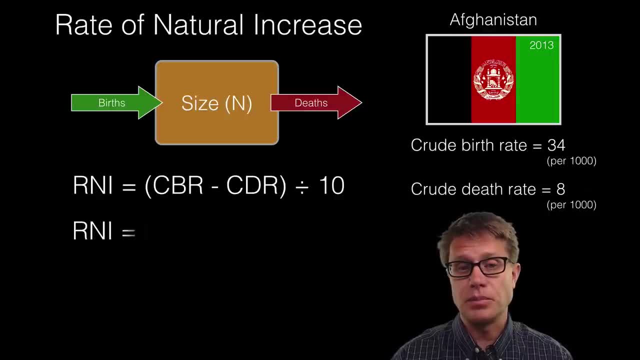 8.. So if we want to figure out the rate of natural increase, we just plug those values in: 34 minus 8 is 26, divided by 10 is 2.6 percent, And so that means this population is going to be increasing over time. Now you could try one with the United States, If I give. 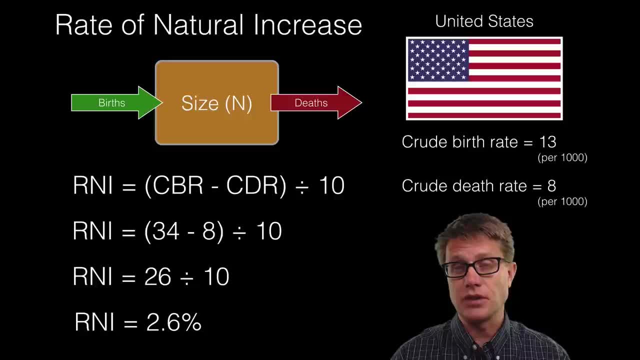 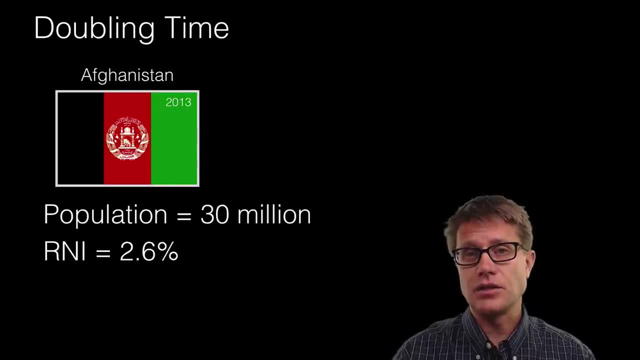 you the birth rate and the death rate? could you calculate that rate of natural increase? I hope so. I will put the answer in the description down below. Now, once we have that value, how much it is increasing- it is very easy to figure out the doubling. 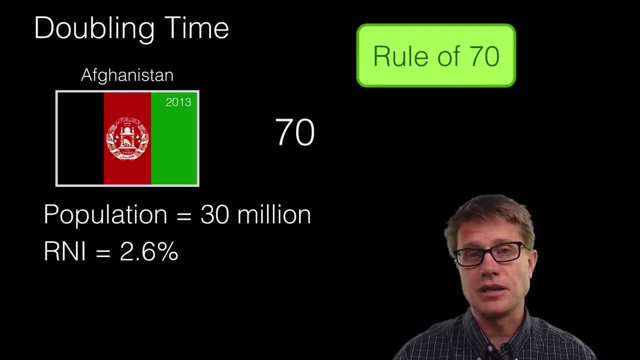 So how do we do that? Remember that rule of 70. You simply take 70 divided by the increased percent, which is going to be 2.6. And then it is going to give us approximately 27 years. So what does that mean? The population in Afghanistan right now is 30 million, So in 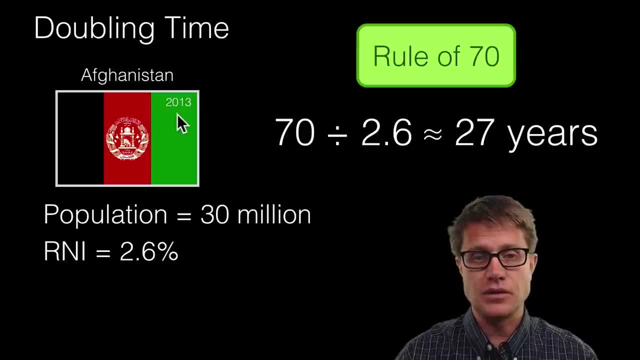 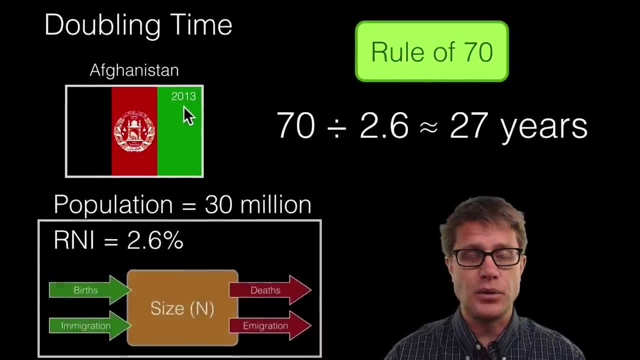 27 years, it will be 60 million. And so, if it is 2013,, right, when these values were given out, it is going to be 2040 when the population goes to 60 million. Now, is that super accurate? It may change over time And I am not. 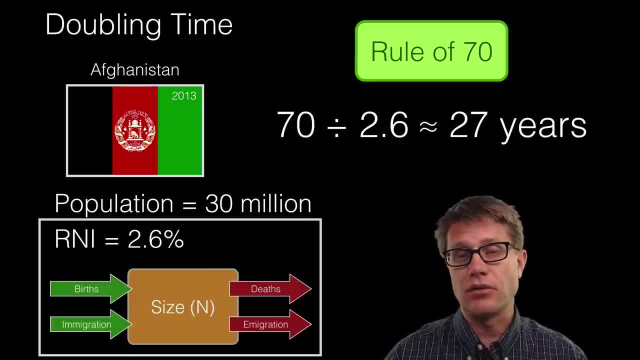 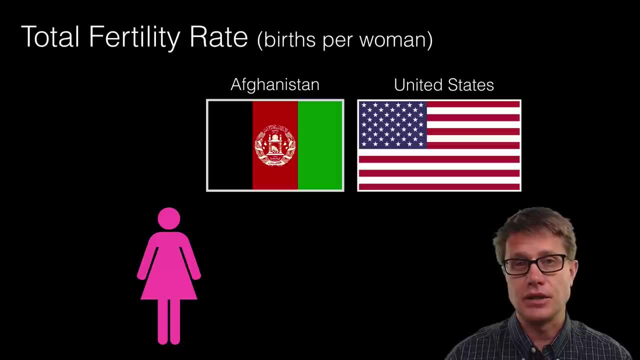 really dealing with immigration and emigration, but it is a simple, powerful tool that you can use. Now, what is changing the birth rate? We call that. demographers call that the total fertility rate. That is going to be the number of births per woman during her reproductive. 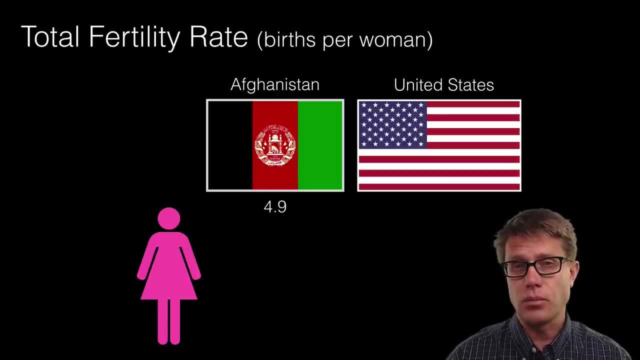 period of time. And so if we look at what it is in Afghanistan, it is 4.9.. So this imaginary woman who is around today will, in general, have 5 children. If we look at what it is in the US, that number is going to be 1.9.. So why do we see such a huge difference between? 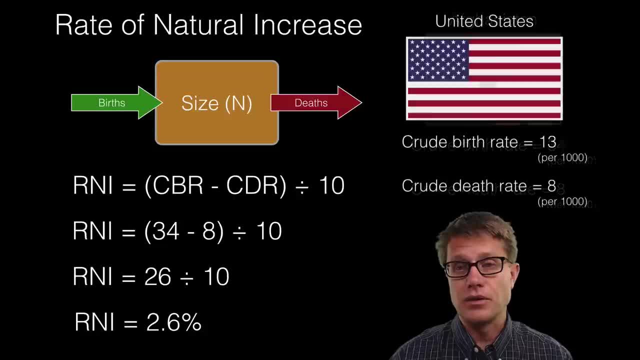 to be increasing over time. Now you could try one with the United States. If I give you the birth rate and the death rate, could you calculate that rate of natural increase? I hope so. I will put the answer in the description down below. Now, once we have that value, how? 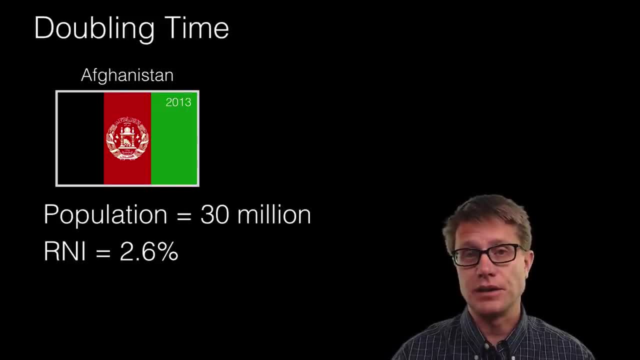 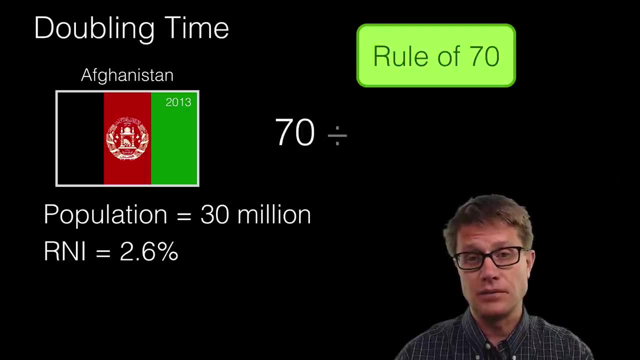 much it is increasing. it is very easy to figure out the doubling. So how do we do that? Remember that rule of 70. You simply take 70 divided by the increased percent, which is going to be 2.6. And then it is going to give us approximately 27 years. 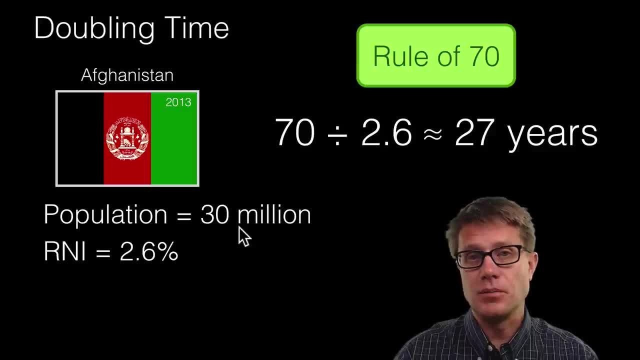 So what does that mean? The population in Afghanistan right now is 30 million, So in 27 years it will be 60 million, And so if it is 2013, right when values were given out, it is going to be 2040 when the population goes to 60 million. Now. is that super accurate? 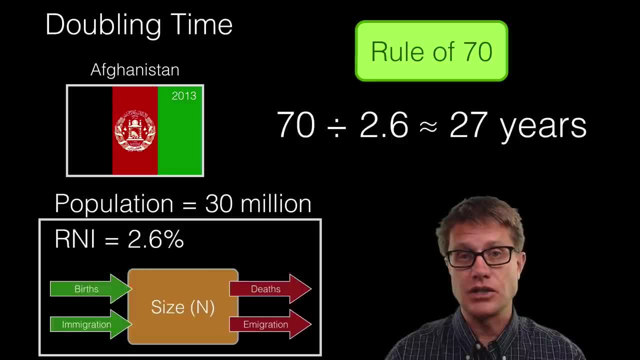 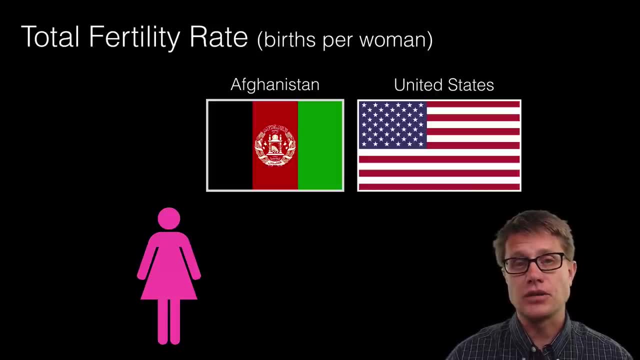 It may change over time And I am not really dealing with immigration and emigration, but it is a simple, powerful tool that you can use. Now, what is changing the birth rate? We call that. demographers call that the total fertility rate. That is going to be the number of births per woman during her reproductive. 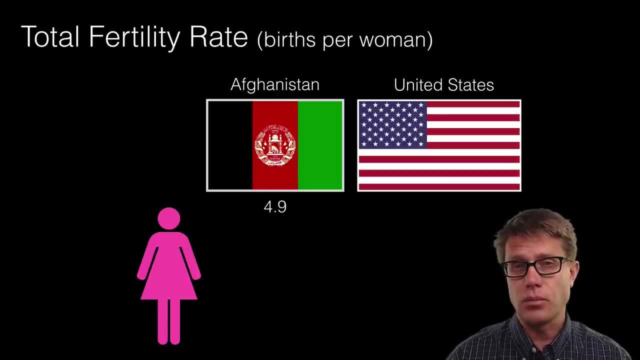 period of time. And so if we look at what it is in Afghanistan, it is 4.9.. So this imaginary woman who is around today will, in general, have 5 children. If we look at what it is in the US, that number is going to be 1.9.. So why do we see such a huge difference between? 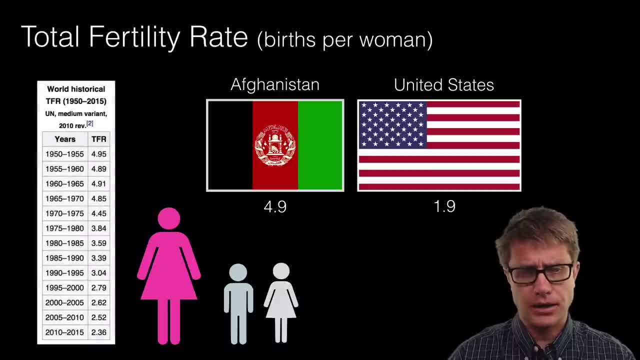 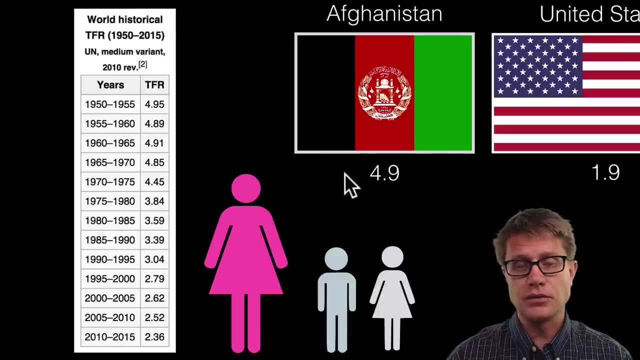 Afghanistan and the US. Well, let's talk globally for a second. So the TFR total fertility rate back in 1950 globally around the world was 4.9.. So it is closer to what Afghanistan is today And you can see that it has decreased over time. So why do we see this decrease? 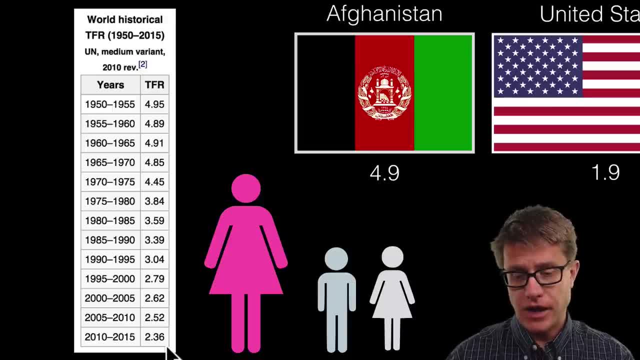 over time. Well, in developed countries, women are going to have access to birth control. They are also going to have access to education. They are also going to have access to education And employment. Therefore, they do not have to get married and start having kids right. 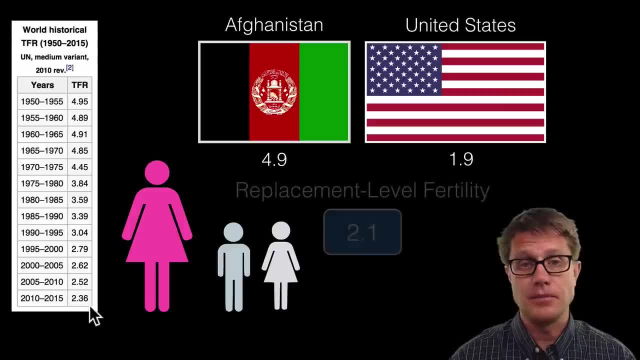 away for stability, So they are going to have less kids over time. Now, a value that demographers will use is called the replacement level: fertility. What does that value have to be to keep our population stable? And so you might think it is going to be 2, because we have the mom. 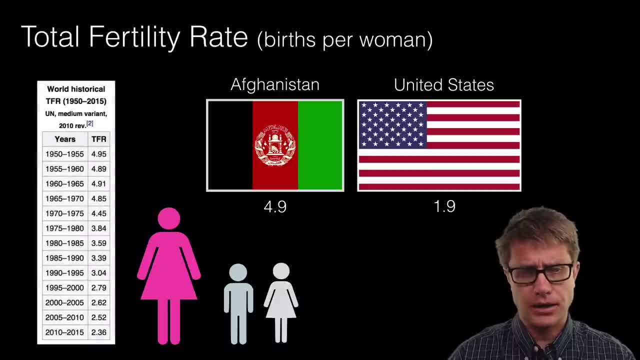 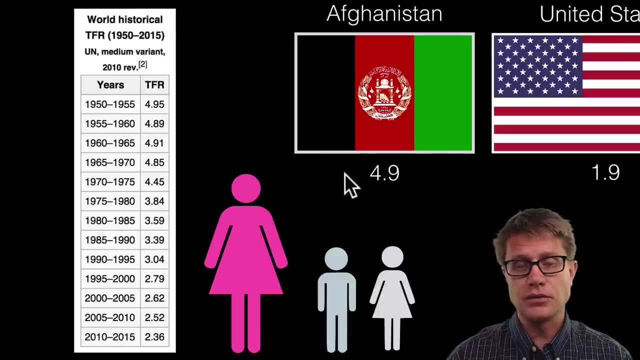 Afghanistan and the US. Well, let's talk globally for a second. So the TFR total fertility rate back in 1950 globally around the world was 4.9.. So it is closer to what Afghanistan is today And you can see that it has decreased over time. So why do we see this decrease? 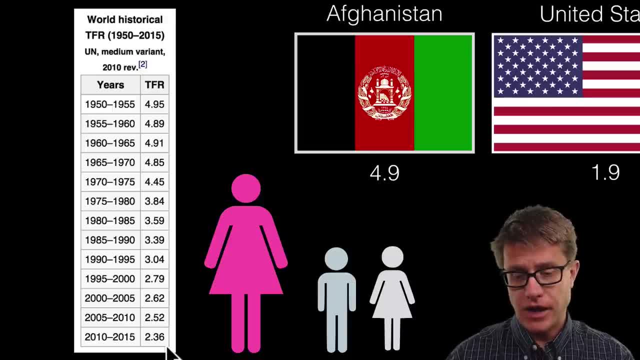 over time. Well, in developed countries, women are going to have access to birth control. They are also going to have access to education. They are going to have access to education And employment. Therefore, they do not have to get married and start having kids right. 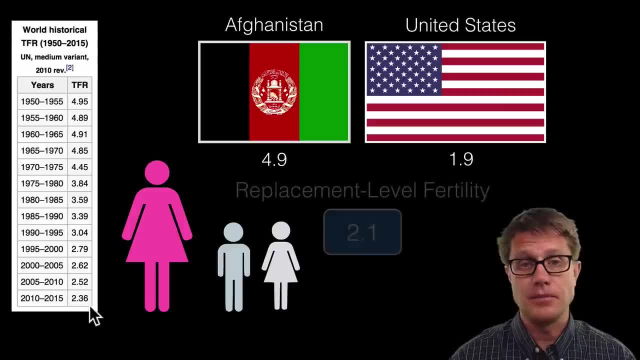 away for stability, So they are going to have less kids over time. Now, a value that demographers will use is called the replacement level: fertility. What does that value have to be to keep our population stable? And so you might think it is going to be 2, because we have the mom. 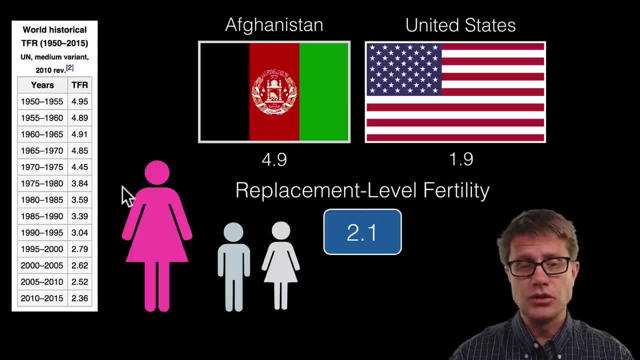 and she has to replace herself and the dad. So you think it would be 2.. But due to mortality rate it has to be a little bit higher, And in developing countries it has to be even a little bit higher than that. And in developing countries it has to be even a little bit higher. 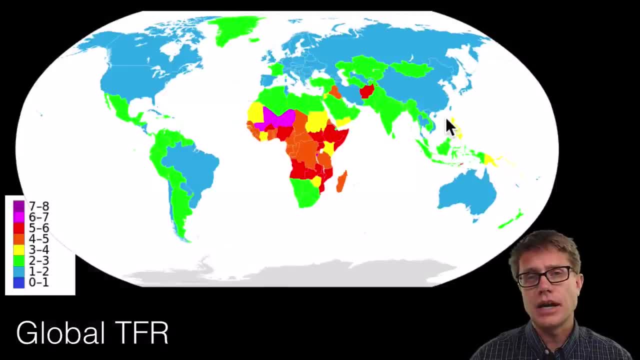 than that To have a stable population. So if we look at those fertility rates, there is going to be unequal distribution. So in the United States the value is going to be between 1 and 2. But in sub-Saharan Africa we are going to see really large values. That. 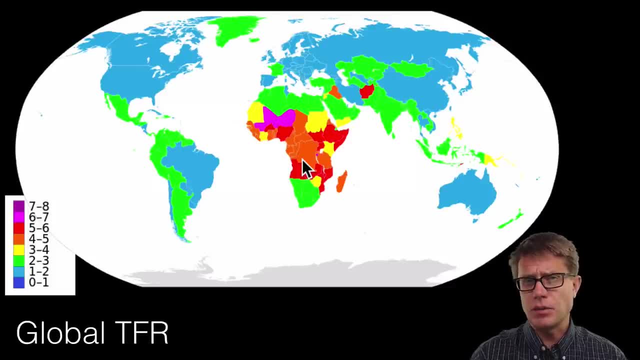 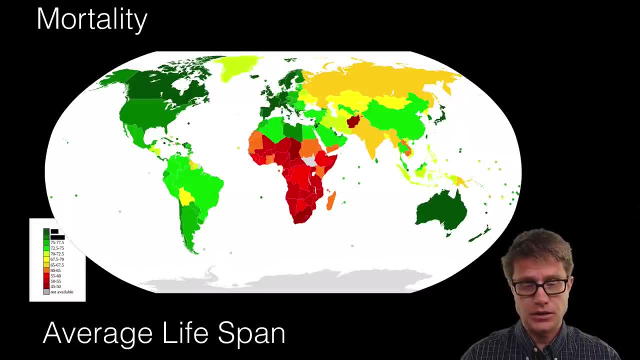 is because a lot of these are developing countries. Now we have only talked about the fertility rate And we have not talked about the mortality rate. So if we look at the average life span in different countries, in a lot of sub-Saharan Africa that is going to be really low, Like. 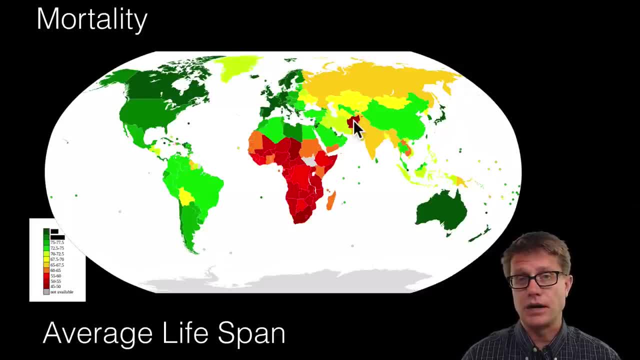 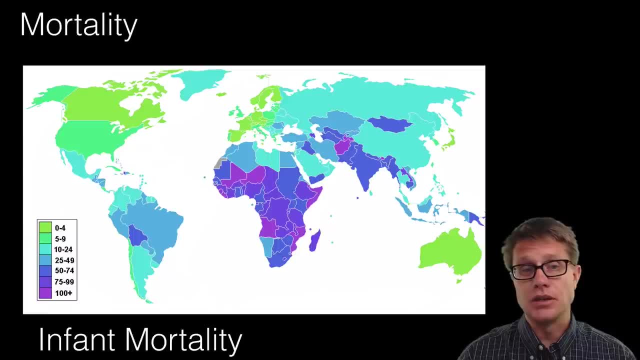 in Afghanistan it is going to be the average person, only living between 1 and 2 years, Only living between 45 and 50. Now disease war can contribute to that. One of the best measures of how developed a country is is the infant mortality rate. So in the US, 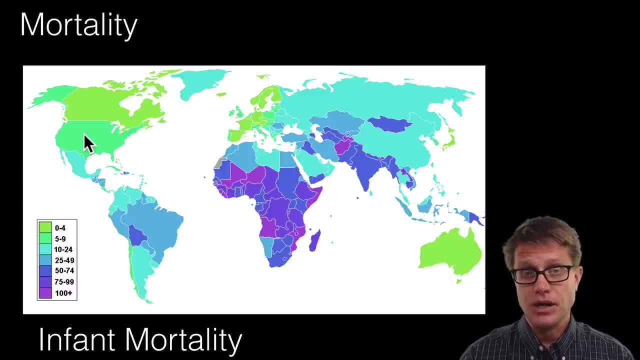 that value is going to be between 5 and 9 per 1000 people, But look at this: In some parts of Africa, that number is going to be approaching 100.. In other words, 1 of 10 infants that are born are going to die, And so what I have been alluding to is this demographic. 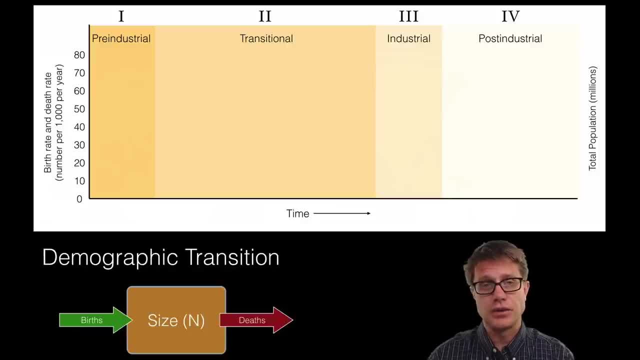 transition. What happens as a country is industrialized, What happens as it goes from a pre-industrial to a post-industrial country And a really good model, is called the demographic transition. So births are going to be in green, Deaths are going to be in red, And so, if we look at the death rate, what happens to the death? 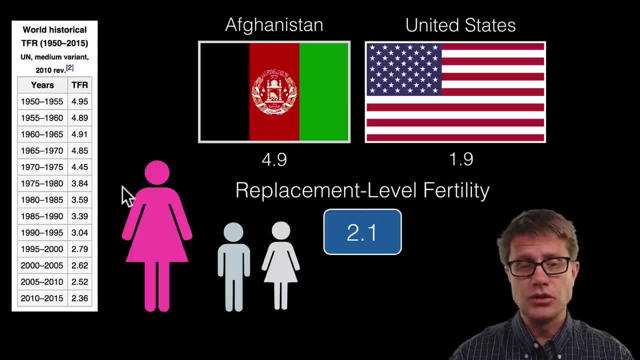 and she has to replace herself and the dad. So you think it would be 2.. But due to mortality rate it has to be a little bit higher, And in developing countries it has to be even a little bit higher than that. And in developing countries it has to be even a little bit higher. 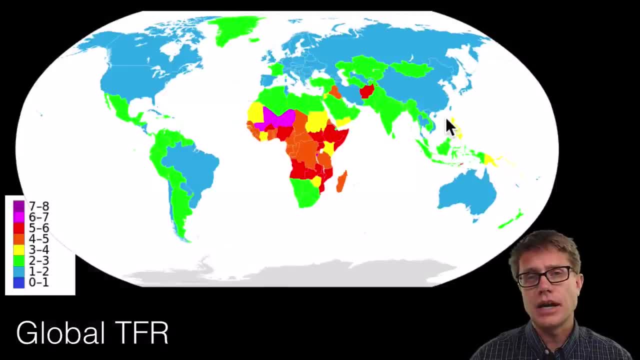 than that To have a stable population. So if we look at those fertility rates, there is going to be unequal distribution. So in the United States the value is going to be between 1 and 2. But in sub-Saharan Africa we are going to see really large values. That. 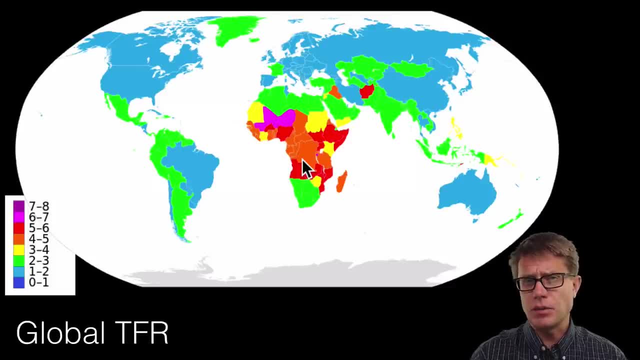 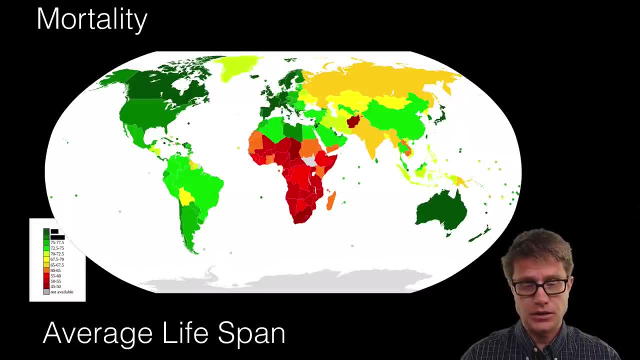 is because a lot of these are developing countries. Now we have only talked about the fertility rate And we have not talked about the mortality rate. So if we look at the average life span in different countries, in a lot of sub-Saharan Africa that is going to be really low, Like. 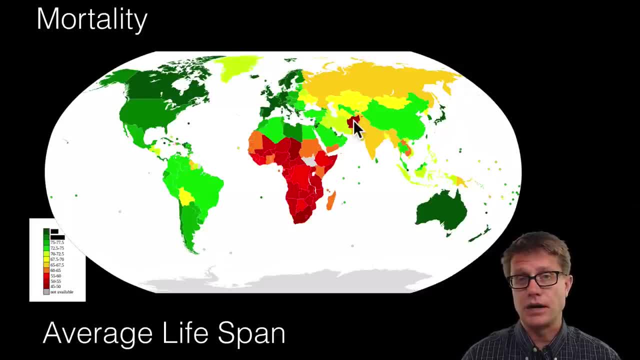 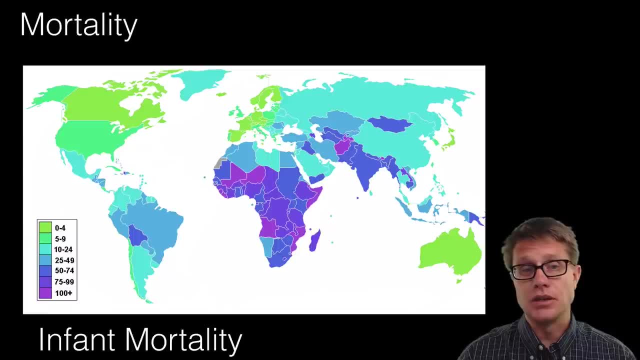 in Afghanistan it is going to be the average person, only living between 1 and 2 years, Only living between 45 and 50. Now disease war can contribute to that. One of the best measures of how developed a country is is the infant mortality rate. So in the US, 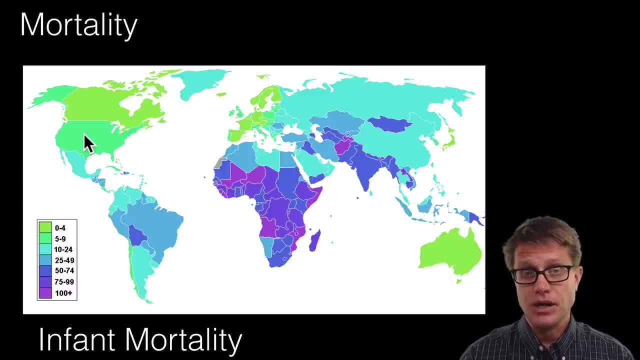 that value is going to be between 5 and 9 per 1000 people, But look at this: In some parts of Africa, that number is going to be approaching 100.. In other words, 1 of 10 infants that are born are going to die, And so what I have been alluding to is this demographic. 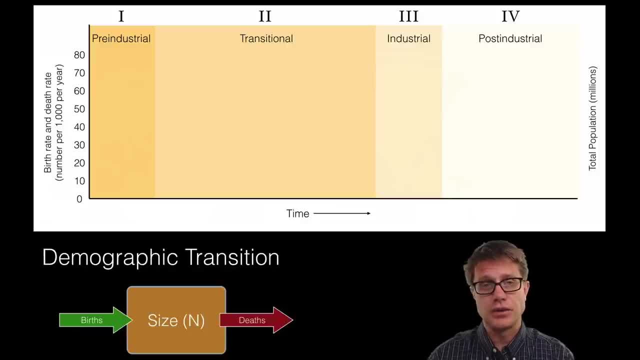 transition. What happens as a country is industrialized, What happens as it goes from a pre-industrial to a post-industrial country And a really good model, is called the demographic transition. So births are going to be in green, Deaths are going to be in red, And so, if we look at the death rate, what happens to the death? 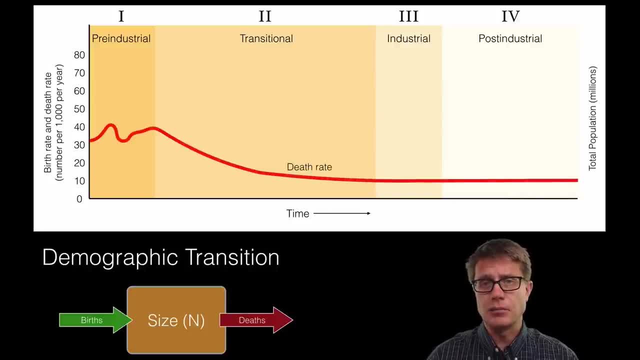 rate during industrialization. Well, it will jump up and down, But eventually what happens is it drops way down and it remains stable. So once we have access to constant food, sanitation, etc. If we look at what happens to the birth rate over time, you will see that it also decreases. 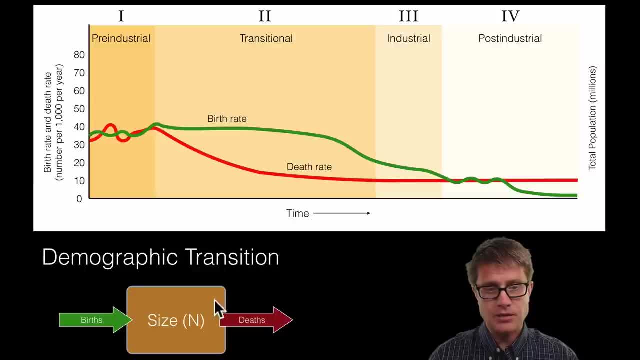 but it shifted to the right a little bit, And so, if we look back at this model of size being increased by births and decreased by deaths, what do you think is going to happen? pre-industrial Well, if these birth and death rates are essentially the same, now they are. 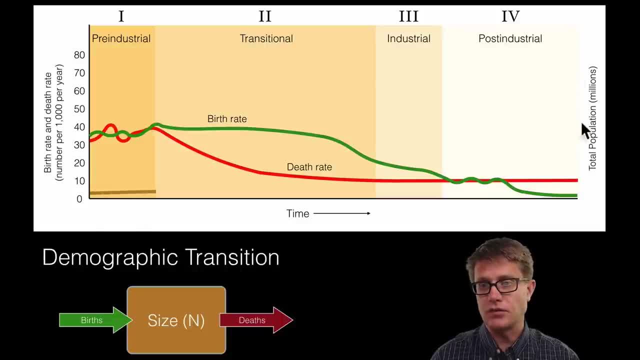 moving up and down. what is going to happen to our population, which I have graphed over here on the right? It is going to remain stable As we move into this transitional period. watch what happens. The first thing that happens is that the birth rate is going to go down. 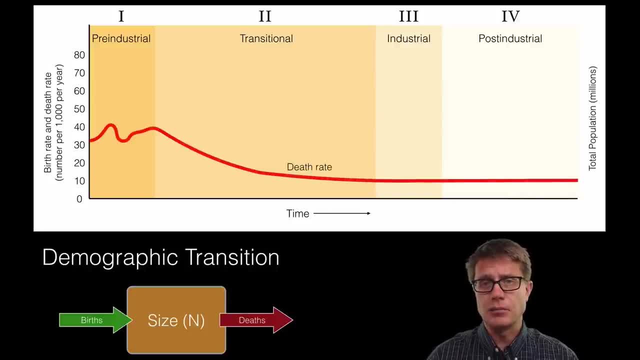 rate during industrialization. Well, it will jump up and down, But eventually what happens is it drops way down and it remains stable. So once we have access to constant food, sanitation, etc. If we look at what happens to the birth rate over time, you will see that it also decreases. 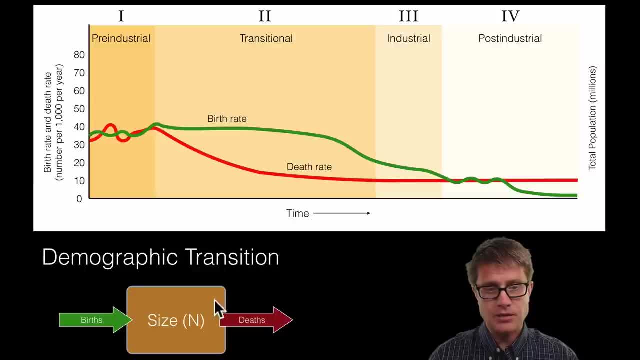 but it shifted to the right a little bit, And so, if we look back at this model of size being increased by births and decreased by deaths, what do you think is going to happen? pre-industrial Well, if these birth and death rates are essentially the same, now they are. 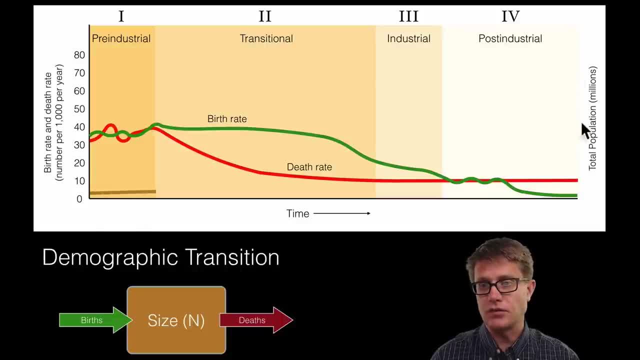 moving up and down. what is going to happen to our population, which I have graphed over here on the right? It is going to remain stable As we move into this transitional period. watch what happens. The first thing that happens is that the birth rate is going to go down. 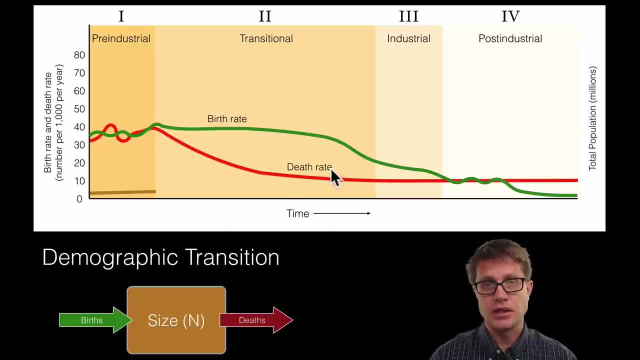 What happens is the death rate will drop off during industrialization, But it takes a while for people to realize that and start having less children, And so it takes a while for the birth rate to drop off. And so if we have a population where the birth rate 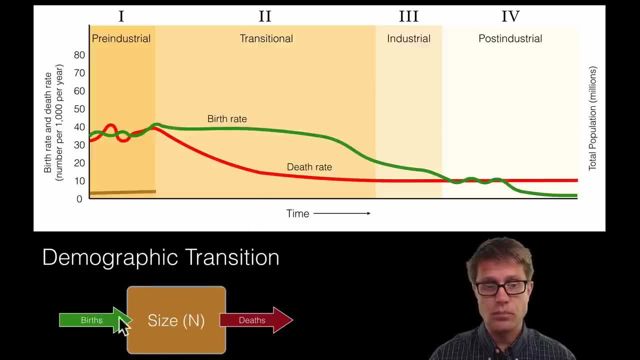 is higher than the death rate. think about this down here. if more births are coming in than deaths are leaving, we are going to see a massive exponential increase in the population. What happens as these two approach each other during the industrial phase? Well, 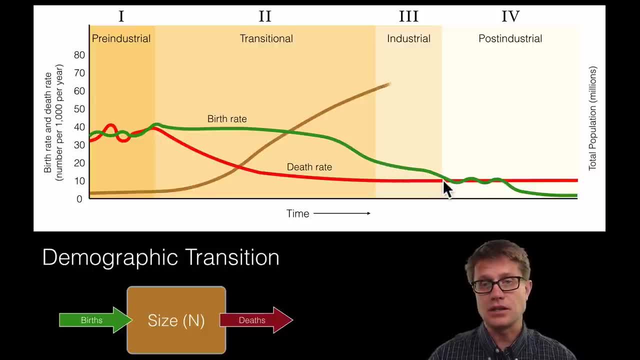 as the birth rate eventually drops to the death rate, you could imagine that it is going to stabilize again. And then what is happening? post-industrial? eventually, we see the population dropping off. So we can see this in a lot of countries Again, it is just. 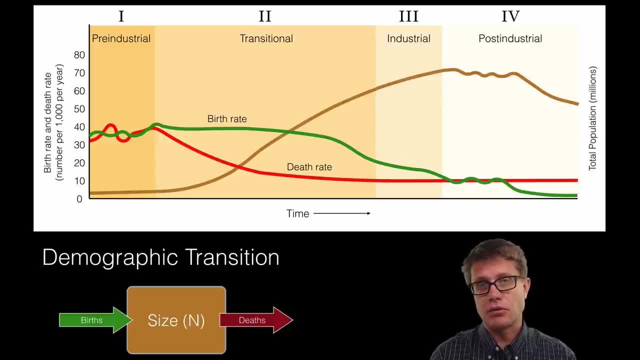 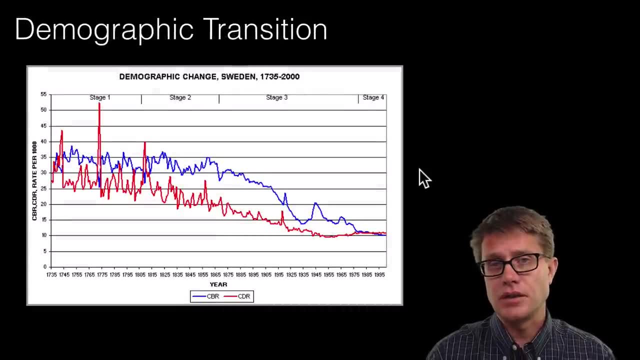 a model, So it is not going to be perfect, But we can look at countries who have gone through this and allow us to make predictions about what is going to happen to countries in the future. So in certain countries we can see the demographic transition occurred. 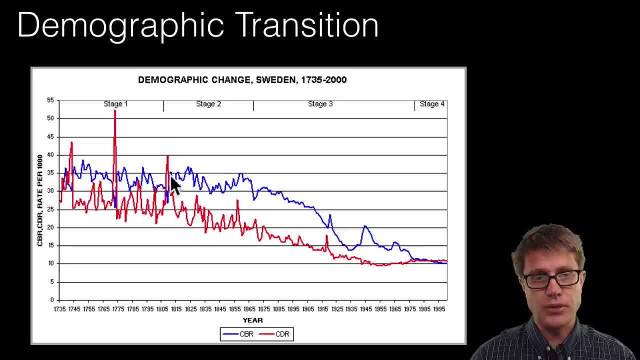 So this is Sweden. What we are looking at here is going to be the birth rates in blue and then the death rates in red. So if we look way back in time in the 1700s, there is a huge increase in death rates. So this was a smallpox outbreak. But what happens over? 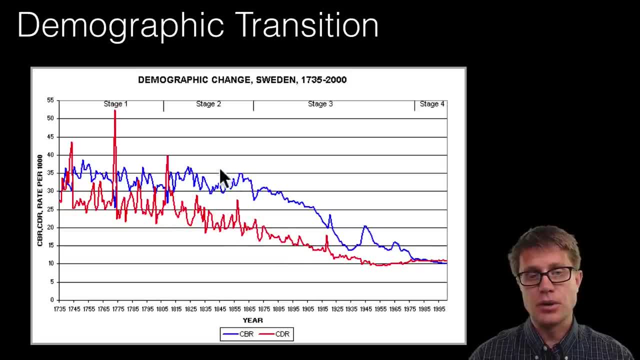 time is the death rate drops off first, and then the birth rate drops off second, And then you can see they reach each other at the same point. So what happened to the population of Sweden during this demographic transition? It increased and then it became stable. A. 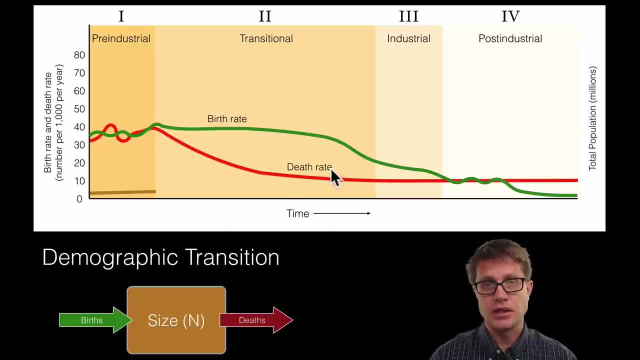 What happens is the death rate will drop off during industrialization, But it takes a while for people to realize that and start having less children, And so it takes a while for the birth rate to drop off. And so if we have a population where the birth rate 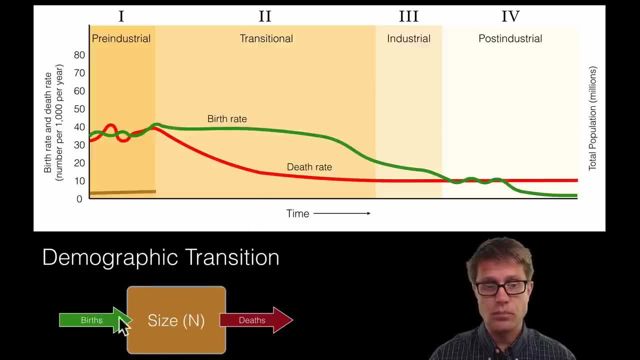 is higher than the death rate. think about this down here. if more births are coming in than deaths are leaving, we are going to see a massive exponential increase in the population. What happens as these two approach each other during the industrial phase? Well, 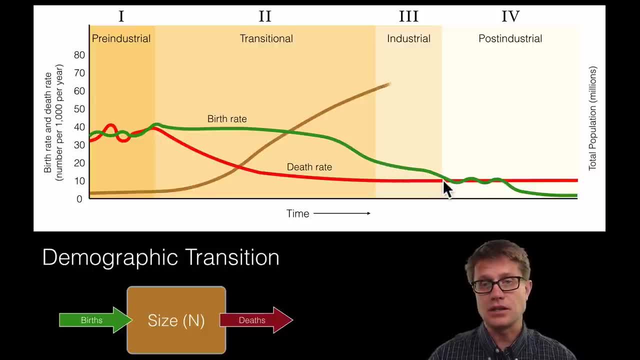 as the birth rate eventually drops to the death rate, you could imagine that it is going to stabilize again. And then what is happening? post-industrial? eventually, we see the population dropping off. So we can see this in a lot of countries Again, it is just. 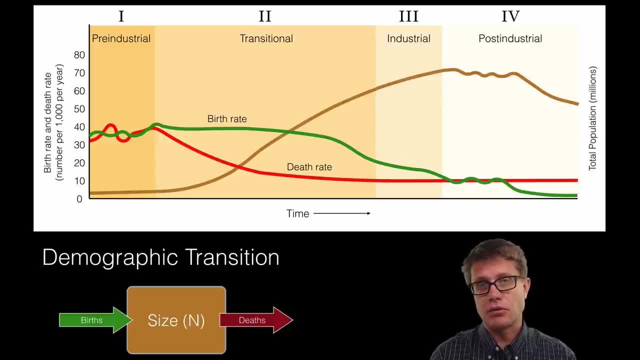 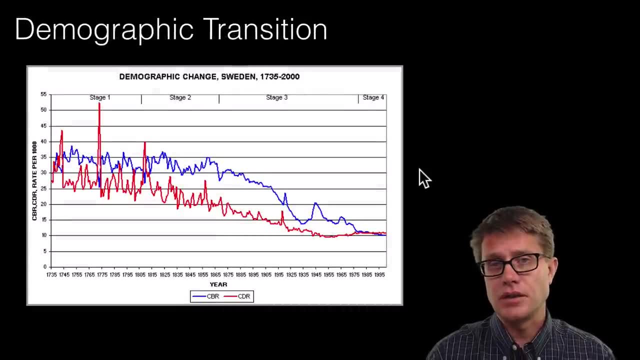 a model, So it is not going to be perfect, But we can look at countries who have gone through this and allow us to make predictions about what is going to happen to countries in the future. So in certain countries we can see the demographic transition occurred. 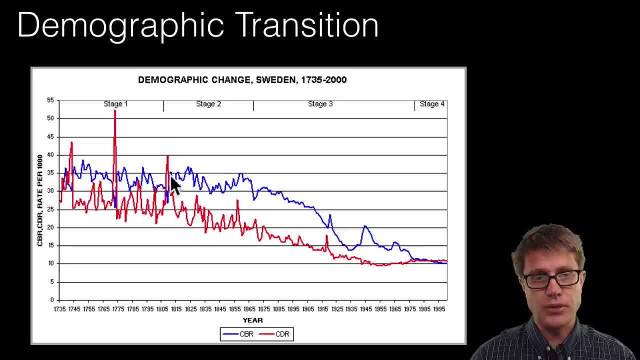 So this is Sweden. What we are looking at here is going to be the birth rates in blue and then the death rates in red. So if we look way back in time in the 1700s, there is a huge increase in death rates. So this was a smallpox outbreak. But what happens over? 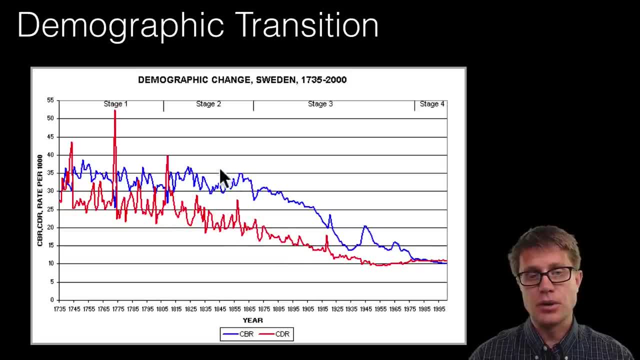 time is the death rate drops off first, and then the birth rate drops off second, And then you can see they reach each other at the same point. So what happened to the population of Sweden during this demographic transition? It increased and then it became stable. A. 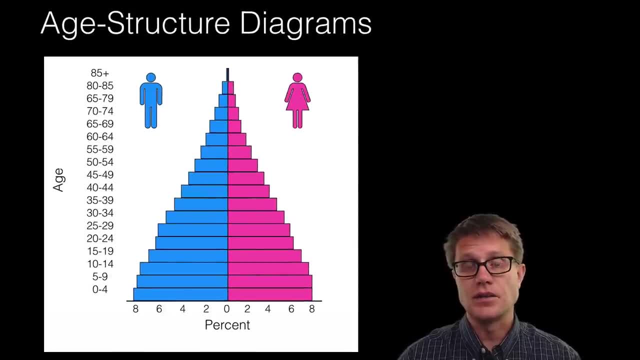 good way to look at where a population is and where it is headed is using something called an age structure graph. So this is an age structure graph, This is an age structure diagram, And so on. an age structure diagram. we will put males on one side, females on. 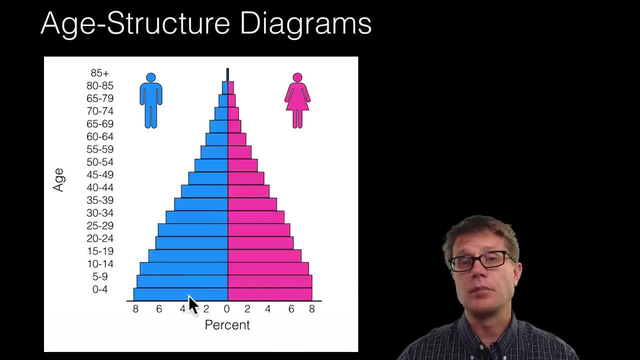 the other, And then the percent they make up of the population, And so if you are a female watching this and you are 18 right now, we could find you right here. So you would be right here. So in this country, you would make up around 7% of the population. 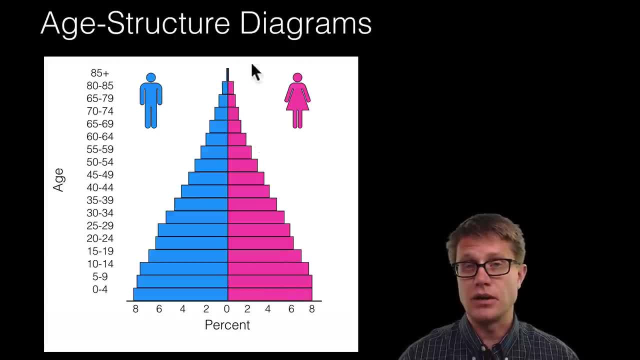 Now, if we see an age structure diagram like this, where we do not have many people that are very old and we have lots of young people, this is going to be a population that is just increasing Just going through that diagram. So this is going to be a population that is. 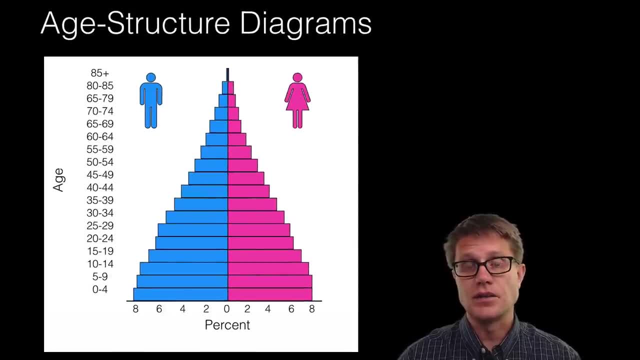 good way to look at where a population is and where it is headed is using something called an age structure graph. So this is an age structure graph, This is an age structure diagram, And so on. an age structure diagram. we will put males on one side, females on. 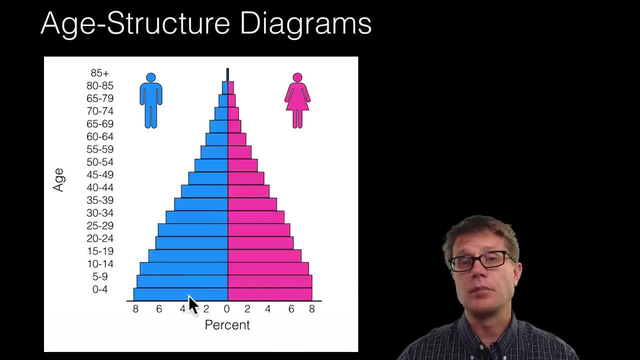 the other, And then the percent they make up of the population, And so if you are a female watching this and you are 18 right now, we could find you right here. So you would be right here. So in this country, you would make up around 7% of the population. 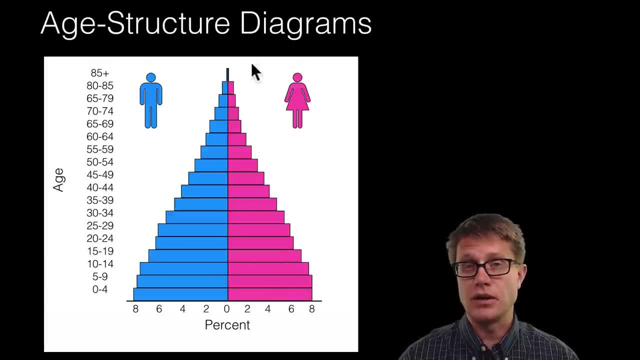 Now, if we see an age structure diagram like this, where we do not have many people that are very old and we have lots of young people, this is going to be a population that is just increasing Just going through that diagram. So this is a population that is just going. 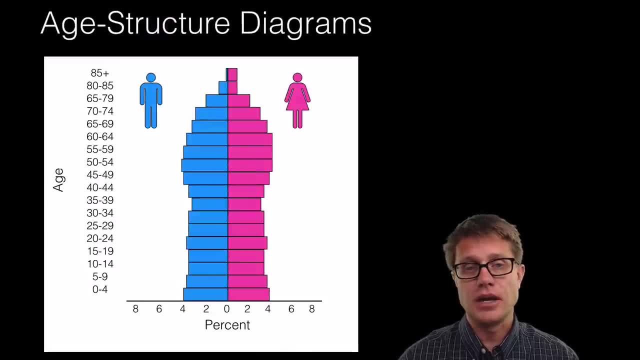 through that diagram, And then we have a population that is just going through that diagram. This is going to be a demographic transition. If, however, we get an age structure diagram that looks like this, where it is pretty much straight on the sides, this is going to be. 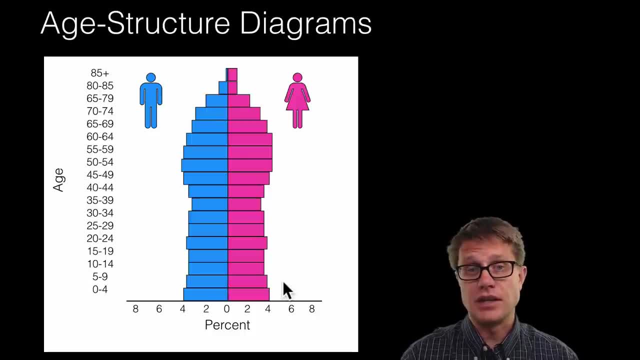 a more stable population. Now this would be what the United States looks like, And you can even see the baby boomers, this large group of babies that were born after World War II, and they are just going to work their way up through the age structure diagram. 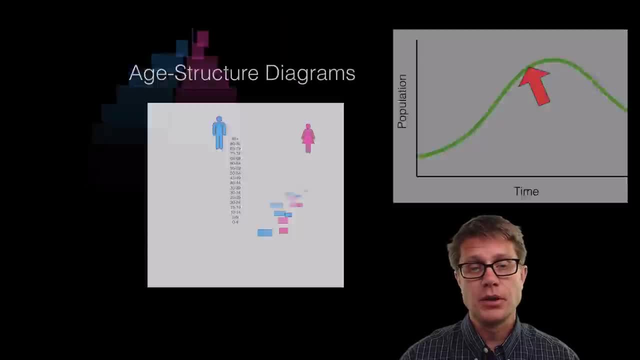 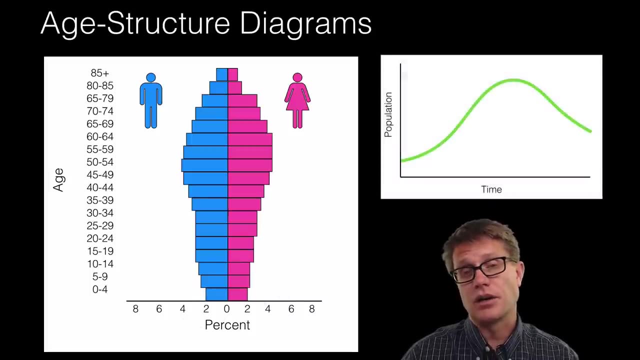 If we look at this demographic transition, where is this going to be Right there? But if we look at a country like Japan, at the bottom we are not going to have many youth at all, And so where is that going to be? We are going to call that post-industrial. Now there are 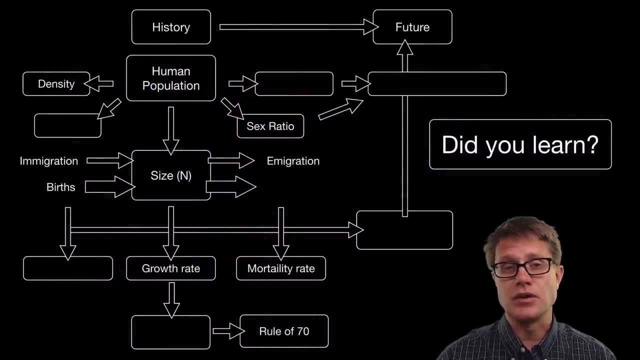 going to be advantages and disadvantages of each of these, but we will talk about those in the next video. And so did you learn the following: That the human population characteristics are: density distribution, sex ratio, age structure, which we can see in an age structure. 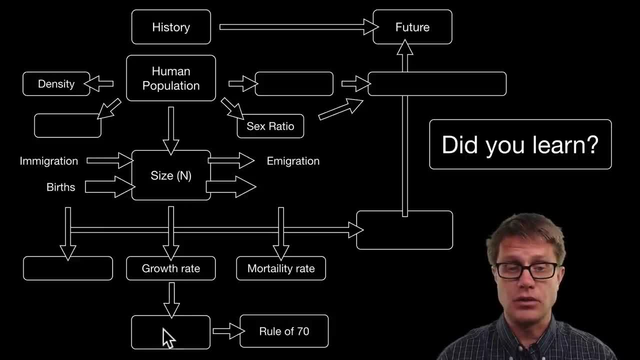 diagram. The size is the most important thing. We can use the growth rate to figure out the doubling time. But what are the other two things that contribute to that? Birth rate and mortality rate, or fertility rate and mortality rate? And then we have the population. 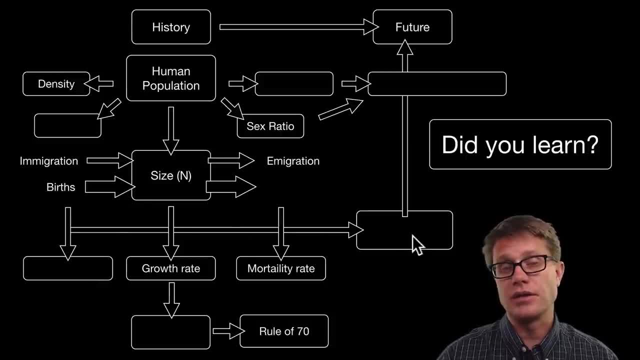 Mortality rate. Remember, industrialization is going to bring about the demographic transition and we can use these two tools to predict the future. We will talk more about what the future holds for humans, but I hope that was helpful.